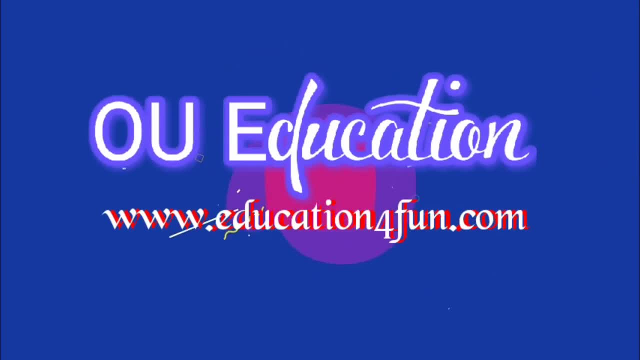 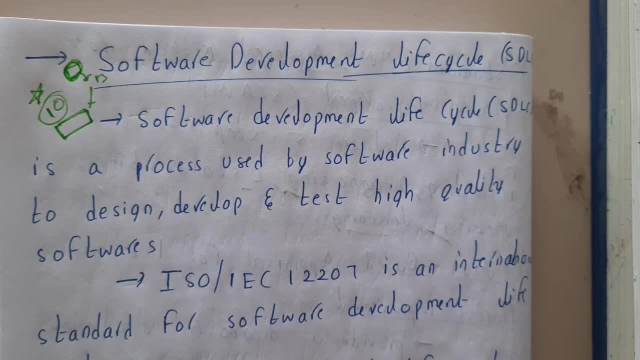 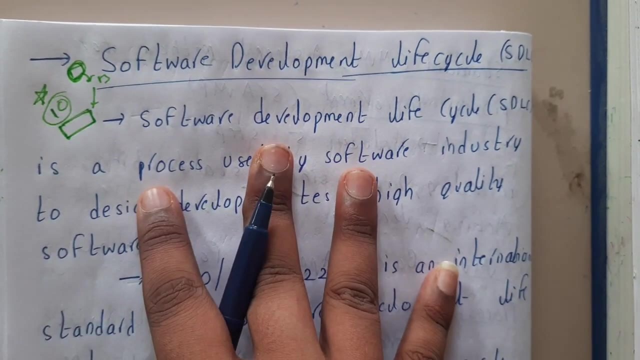 Hello, guys, we are back with our next lecture. In this lecture, let us go through software development life cycle. Guys, the only request that I am requesting you is that, basically, from this lecture onwards, around till 10 lectures, we will be continuing the same process, but 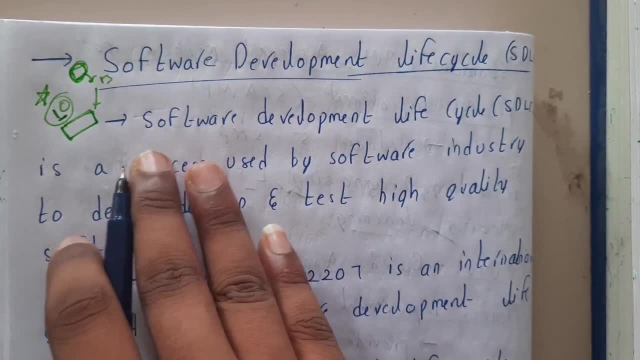 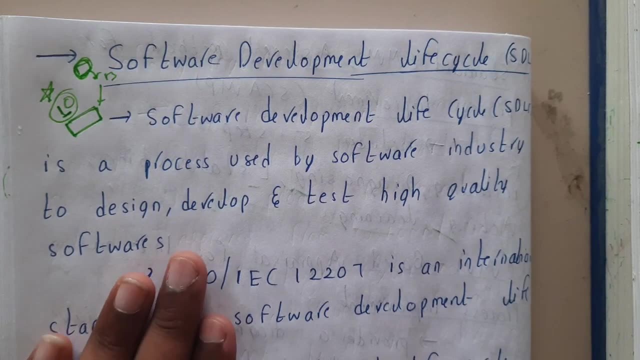 with different models guys. So the process will be the same, like steps will be the almost the same. So I just wrote the theory here perfectly in this question. I wrote the theory perfectly like step by step everything, and in the next 10 lectures we will be just going. 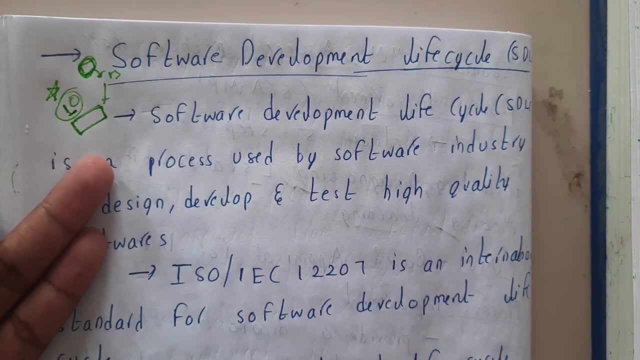 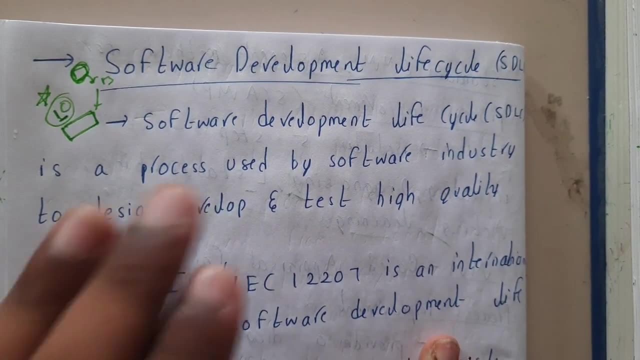 through the overview and the diagram and I will be explaining you in some words. that's it. So if you want theory for the next questions, this video will help you guys. So here the complete, almost the complete, theory has been written. Any additional points are written. 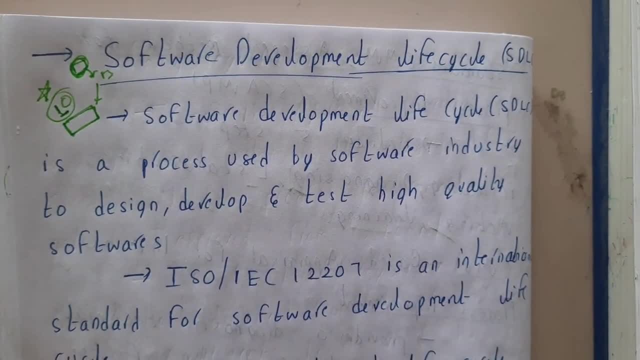 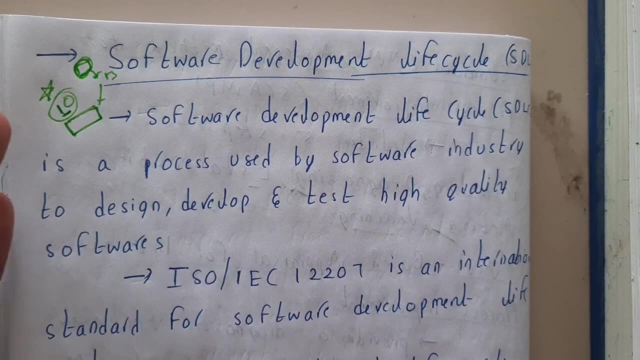 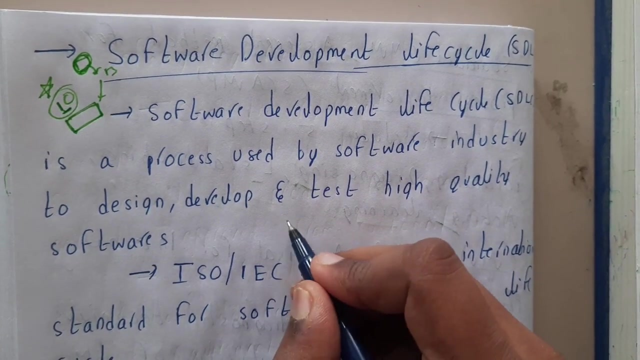 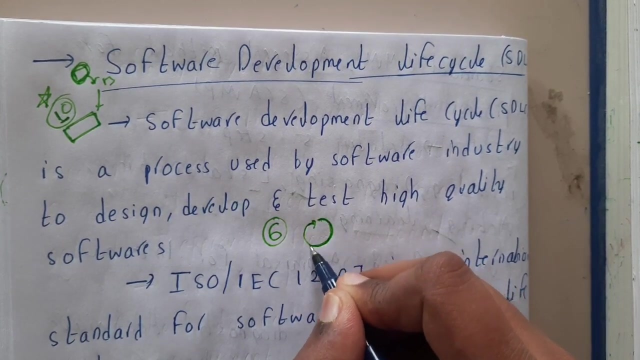 in that particular sessions only. So now let us start with software development life cycle. So you can say that these are a six step process, guys, and this is a loop process. So this is an infinite loop which will continue forever. you can say that Until the agreement. 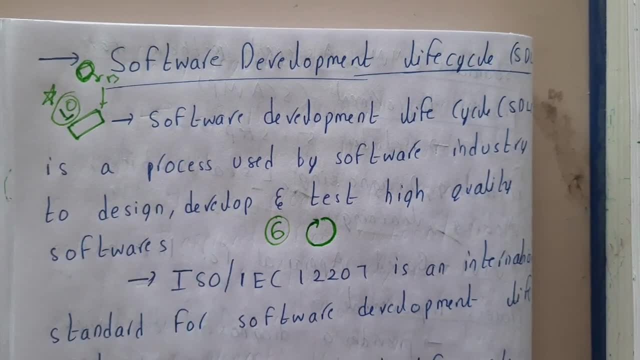 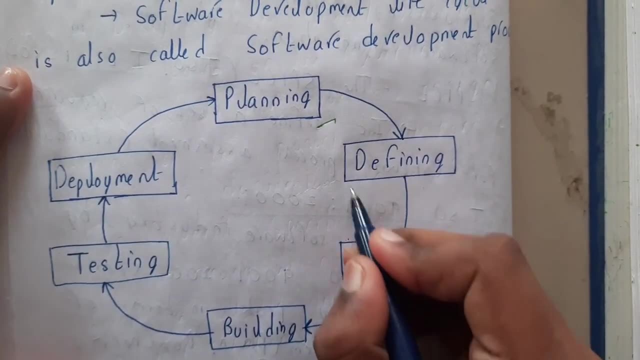 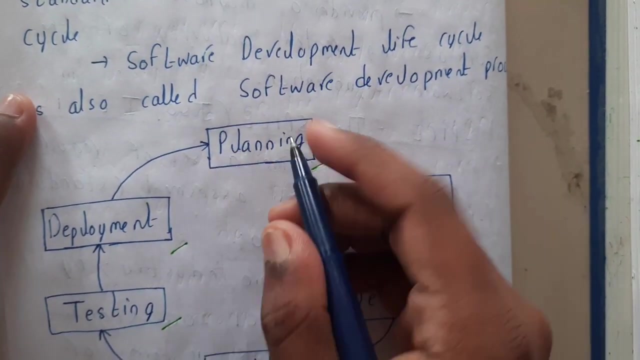 between the company and the project Until the client and the project. So basically, this is a six step process. So the six steps are Planning, Defining, Designing, Building Testing and Deployment. Okay, So planning, Planning is nothing but what you will be planning, guys. So basically, your client will be coming. 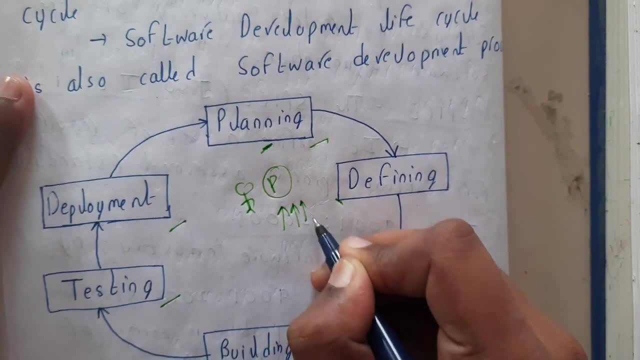 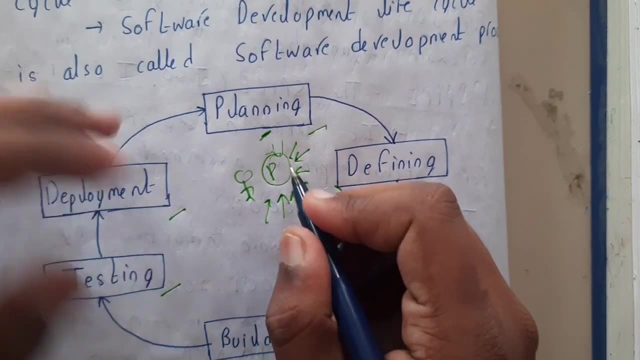 up with a problem. So you will be asking your client about his requirements. So what do you want? What is that? What are you expecting? What is your requirements? You will be asking him continuously all the questions and you will be taking a note of all of them. Okay, 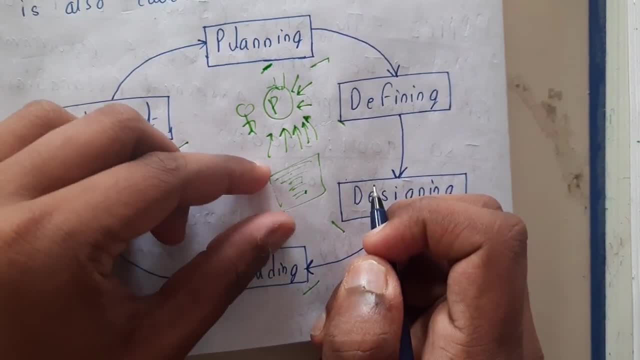 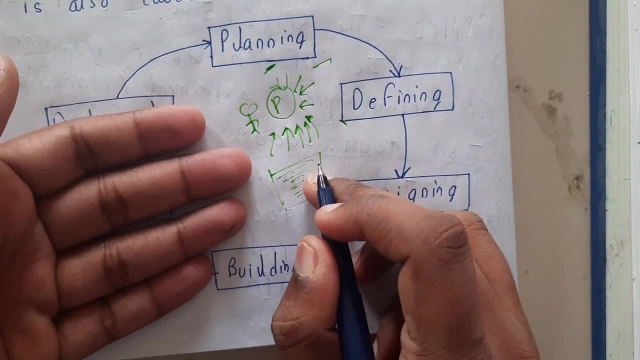 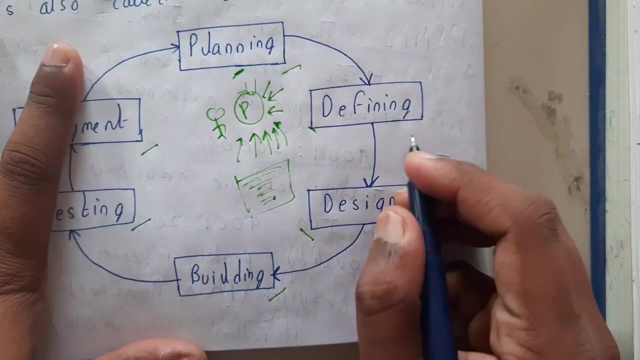 All the answers and you will be analyzing them, guys. So basically, here you're planning and understanding what is the problem or what I am solving, basically So that you will be deciding here. So once you've got an idea that what is the problem and what is the solution that you're thinking to solve it, Then you will be moving on to. 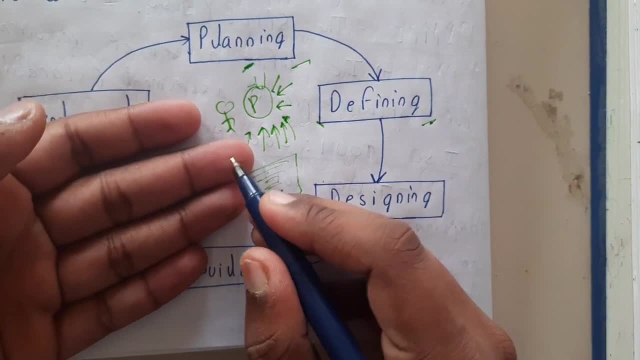 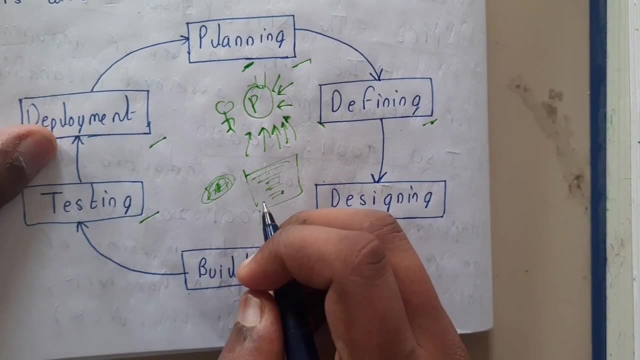 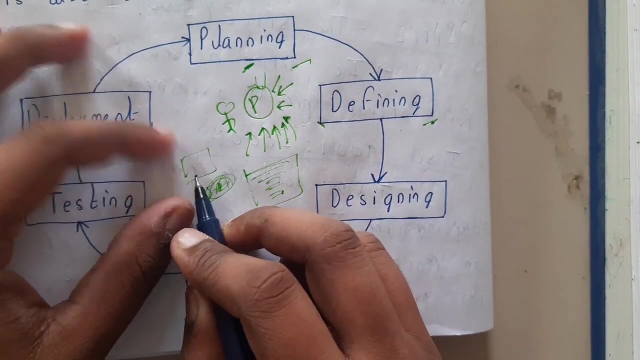 defining guys. So defining is nothing. but here you will be creating the software SRS, as they will be saying: right, software requirement, okay, So they will be analyzing the software requirements and they will be just making a document, Okay, okay. so they'll be making a document and they will be designing it and they'll be planning it here. 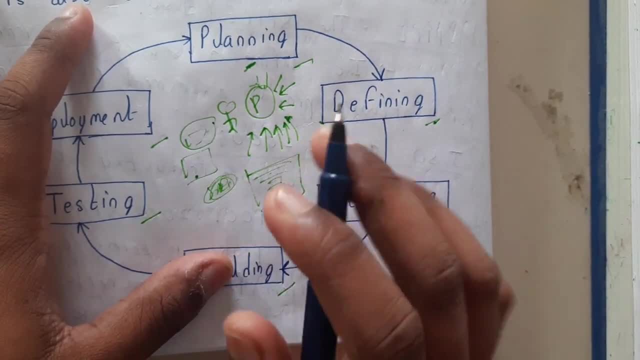 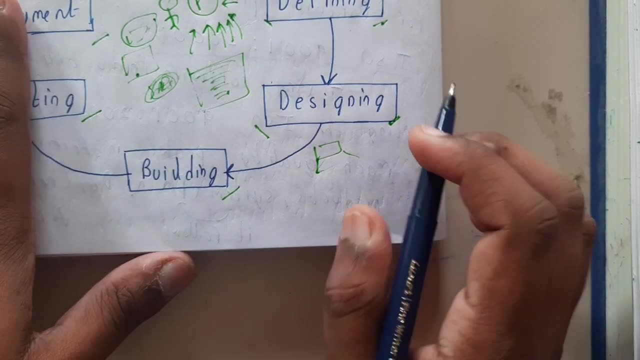 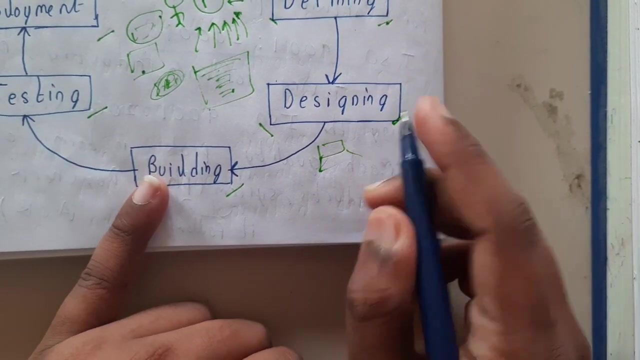 guys, okay. so here they are, having a clear idea what to do. now, in the next stage, they will be designing it. so basically, before building, so let us assume you want to build a house, guys, okay. so when you are building, assume that you want to build a cardboard house- okay, so you will be. 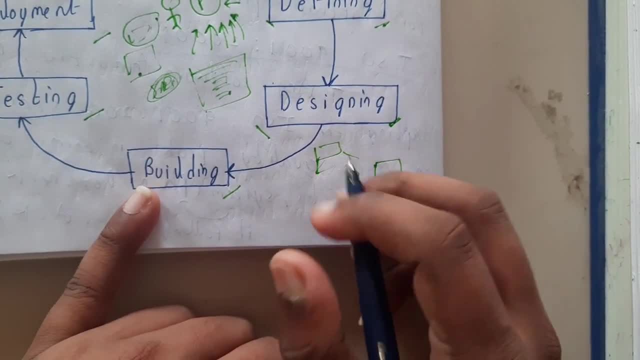 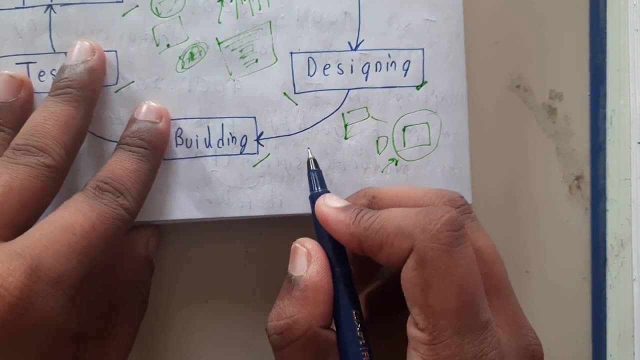 directly taking some carboards and you'll be connecting them, okay, while doing only you'll be analyzing it without any issue. so previously the software developers used to do in this way, but whereas in soft. so you want to assume you want to build a huge building like five floors building. 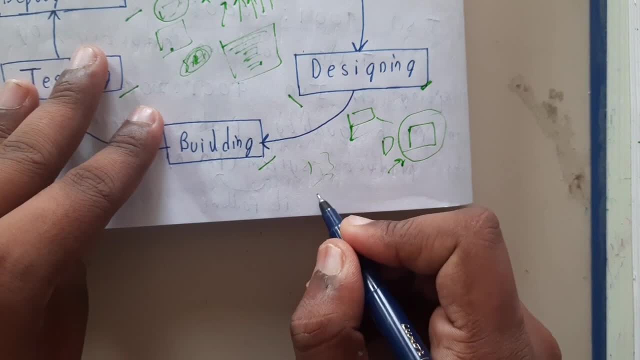 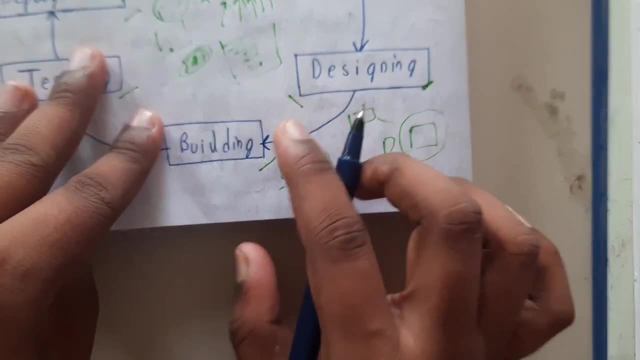 or an apartment. will you directly go and start building guys? no, right. so initially you'll be planning it how the rooms should be, how many floors or how many houses will be in each floor. like you'll be planning it right. so you'll be making a dummy model in your system, or? 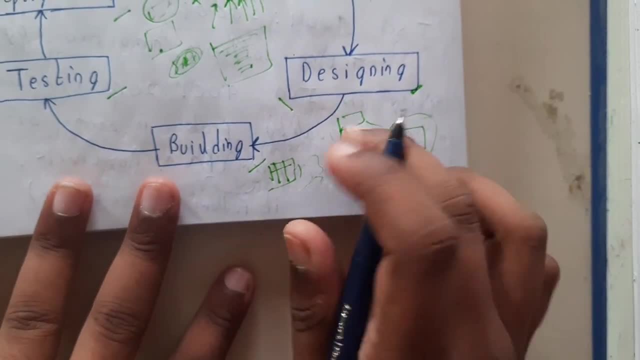 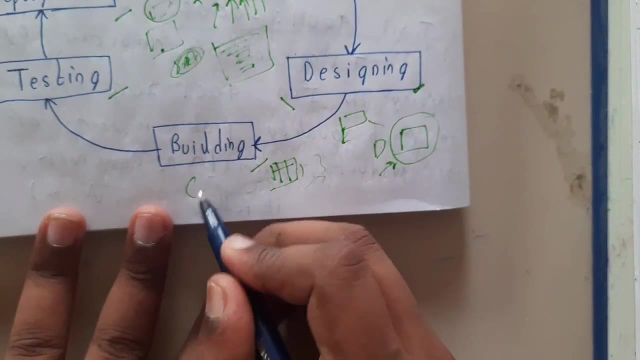 on a paper, right, or a 3d model for it, right. so that comes under designing. so here you'll be designing what will be the output. so once the designing phase is done, you'll be going through building. so building, you can say that it is nothing but coding stage. so you'll be coding the whole project and you'll 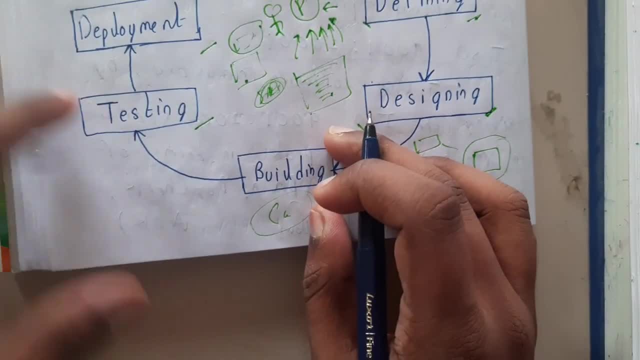 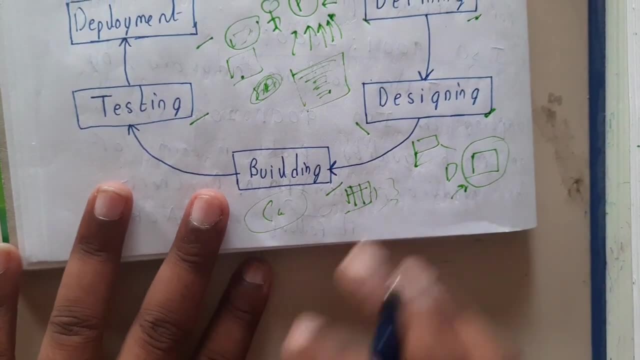 be finally finishing the project in this stage. so once the finishing of the project is done, you will be doing some small, small tests, right guys? like when you code. you'll be doing some tests like whether the program is working, working properly or not, like that, okay. so once it is done, 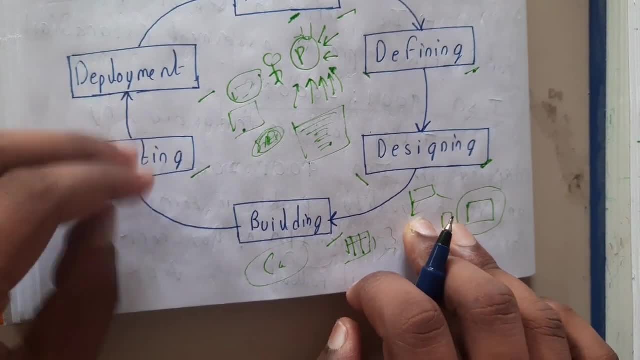 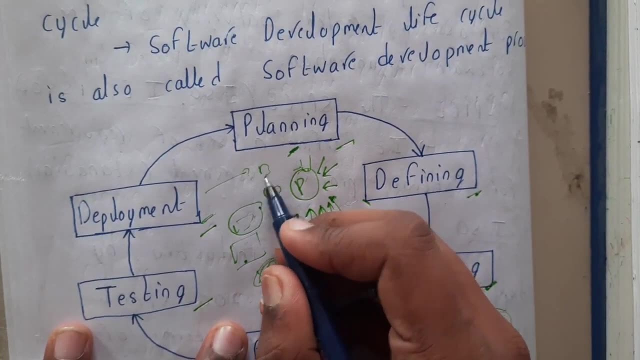 you'll be going through the testing stage. this is the last to second stage going fifth stage. so you'll be doing the testing. so once the testing is done, you'll be going to deployment. deployment is nothing, but you can assume that you'll be providing it to the client and you'll be deploying it to the whole. 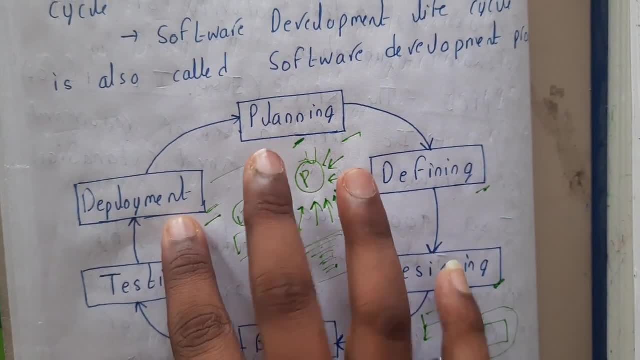 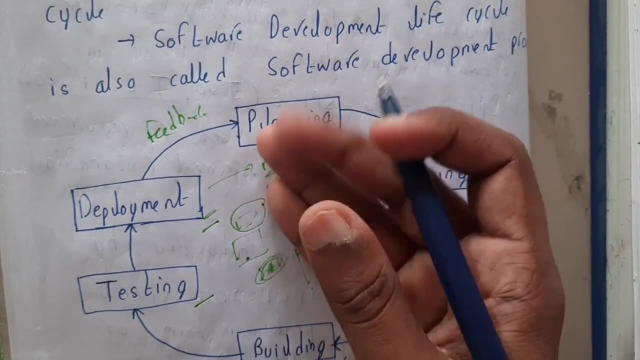 world. okay. so once the deploying is done, so based on the feedback, again, you'll be going to planning. so, based on the feedbacks- like bugs reported and everything you need to solve them right, so you'll be going on to planning again. so this is the software development life cycle. so this is how. 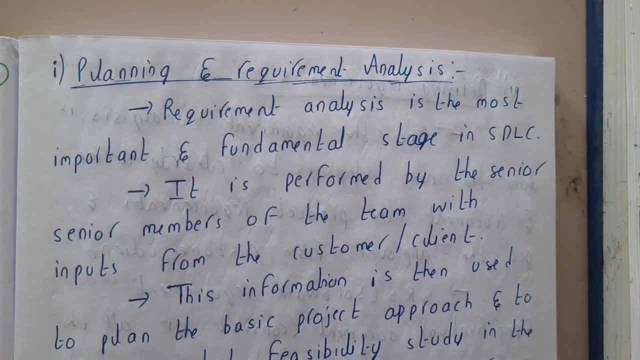 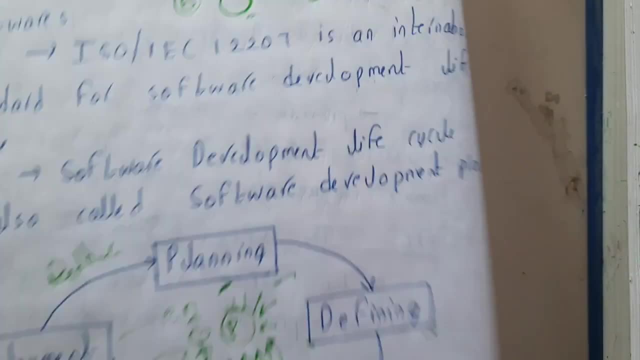 it works, guys. okay, so now let us go through some theoretical points so that it will be clear for you. okay, so planning and requirement analysis both comes into one place, guys, so you can here, you can write planning and requirement analysis. that will be better. okay, so requirement analysis is the most. 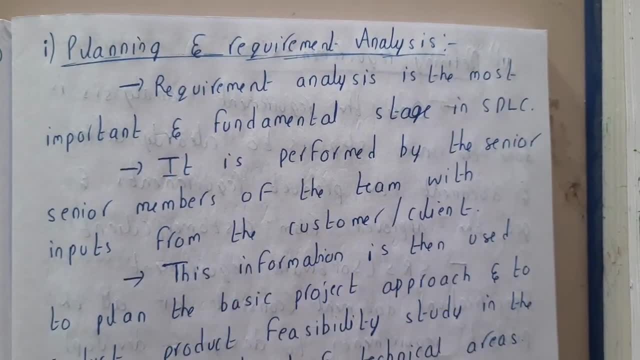 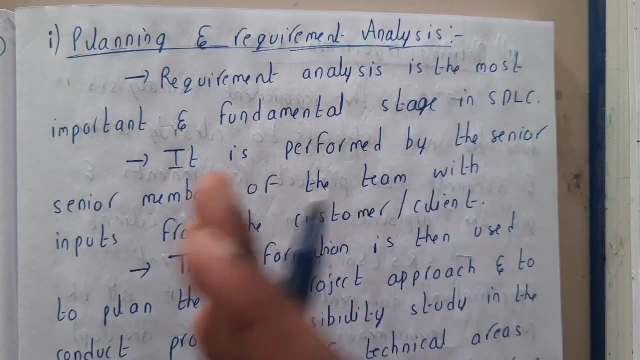 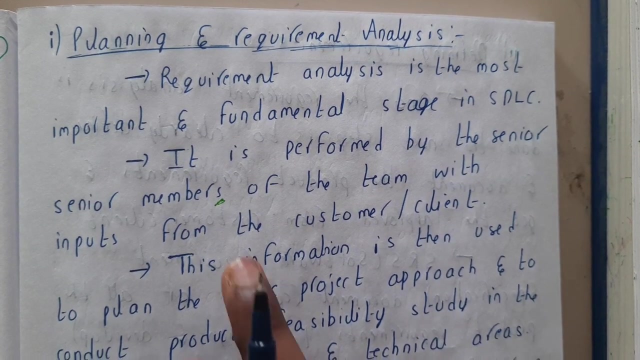 important and fundamental stage of a software development life cycle. i'll be just going through the theoretical points, guys. okay, so it is performed by the senior members. so basically, here you, if you are a new to the company, you will not be going for the requirement gathering some senior employees who are having much experience in projects. they will be going here. 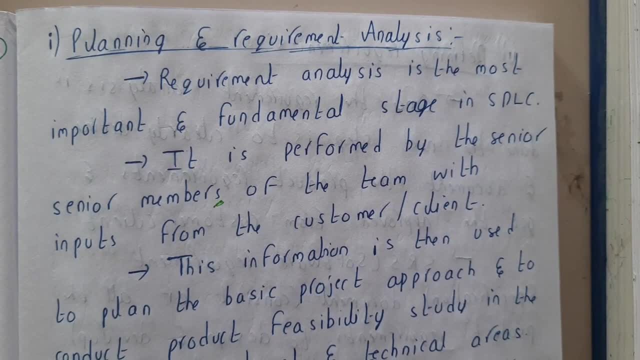 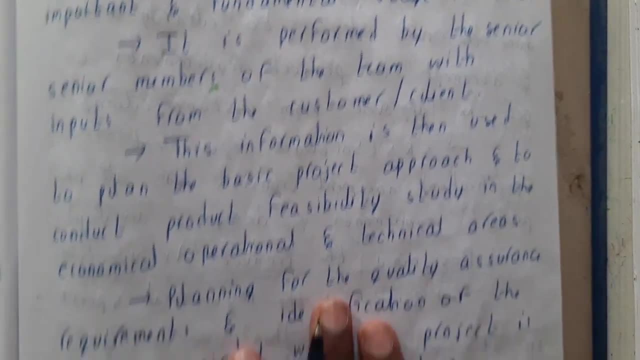 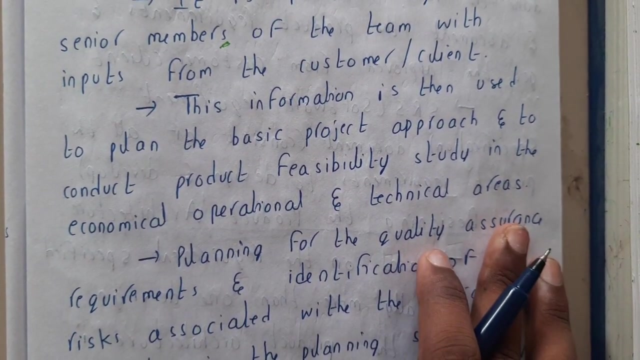 because they will be having a clear idea, right. so what are the things that they should ask? everything they will be having a clear idea. okay, so this information is used to plan the basic project approach and conduct feasibility studies in the economical and operational technical areas. so, basically, if i ask you that, 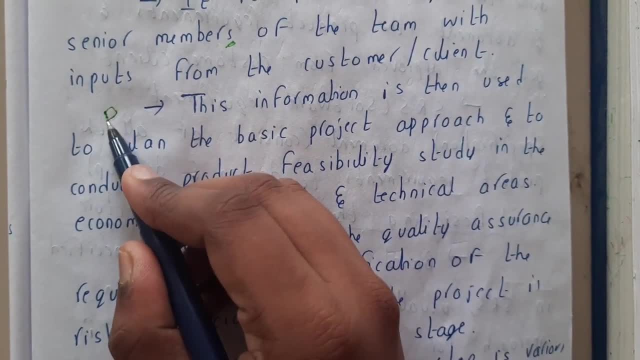 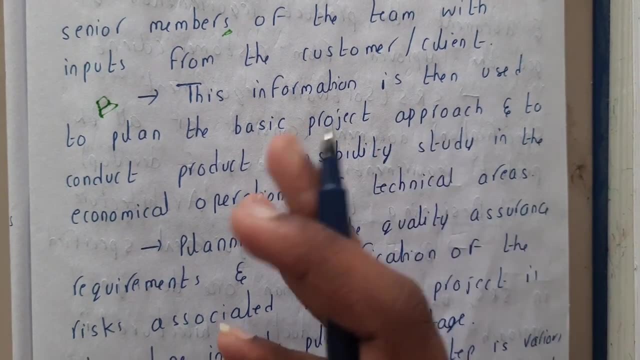 if i ask you to write a project or to a to a project to send- to send a rocket to mars or to send a satellite to max or something to mars or somewhere else- you directly say that okay, that is possible, i'll be doing it like that. you'll be saying no. 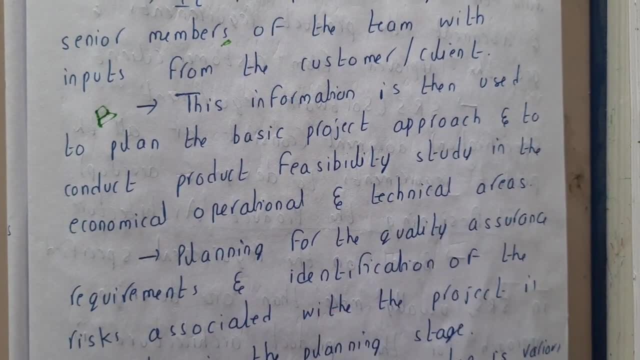 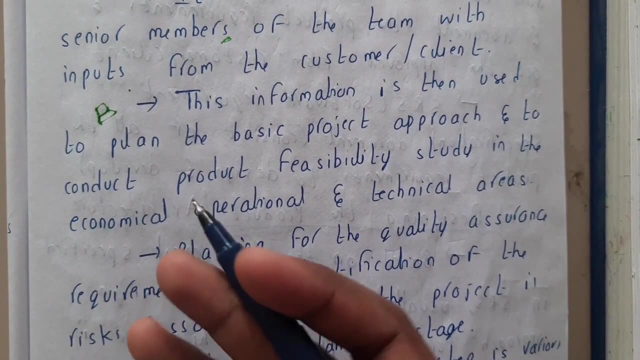 you'll be just first analyzing it whether it is possible or not. what he's saying is it possible or not? or assume that i want to make a pen which is of infinite ink. okay, that idea is funny, right. so, basically, but if you go with this approach, they will be saying that this idea is not feasible, like: 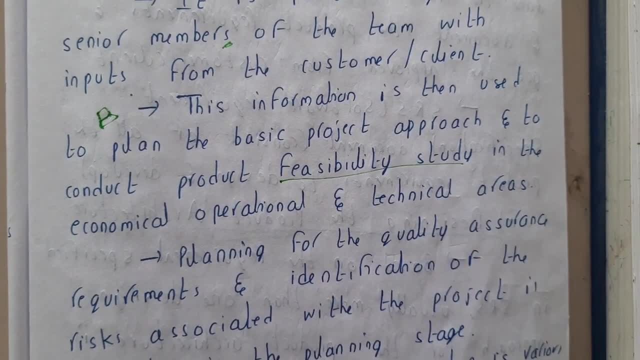 it is not possible in that way. so that is the reason why you need to do some feasibility tests first. okay, so after that you will be planning for the quality assurance of requirements. so basically, are the requirements are enough, or are there even enough benefits, requirements, requirements of this. 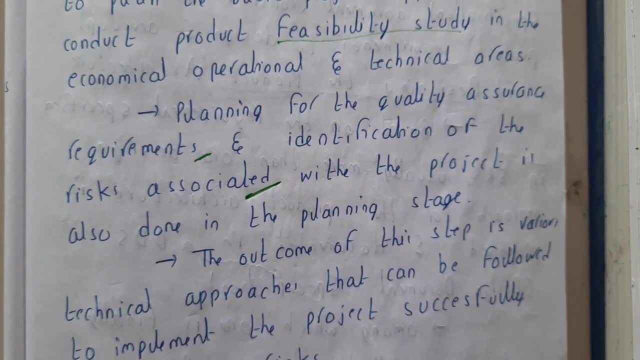 somewhere, state type test. 먼저 you to plan for the quality assurance of requirements. there we will Lori elements of requirements. so basically, these small states like the Step. Would You Do math? you wll be seeing these, Or are there any risks associated with the project? 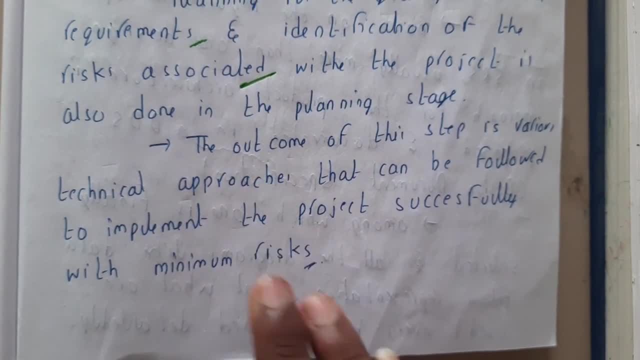 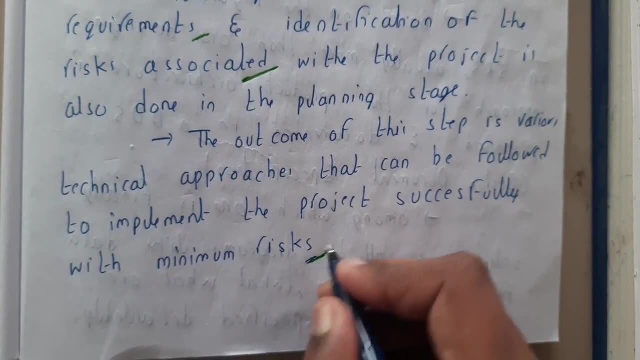 Like that. you will be analyzing them. So at the end you will be. the outcome of this step will be that various technical approaches that can be followed to implement the project successfully with minimum risk. So the outcome of this whole step will be: you will be getting some multiple processes, guys. 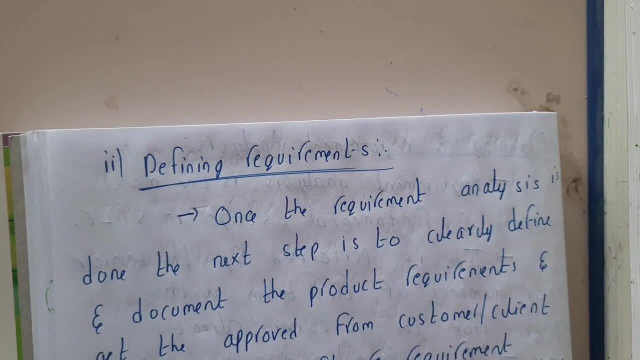 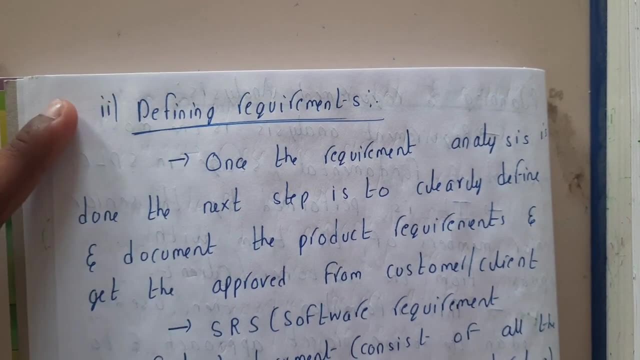 Okay, So basically in the next step, that is nothing but defining requirements. So in this step you will be finalizing the requirements, like how you want, what you want and what is the output that the consumer can expect or the client can expect. 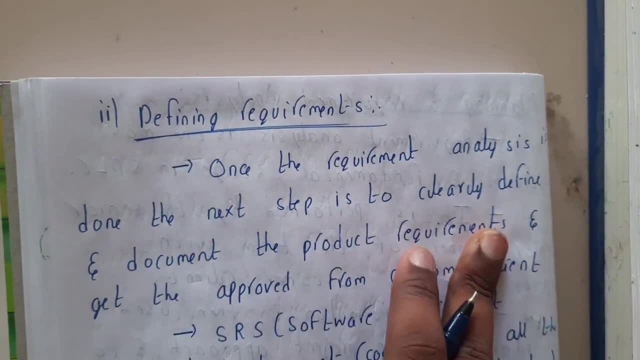 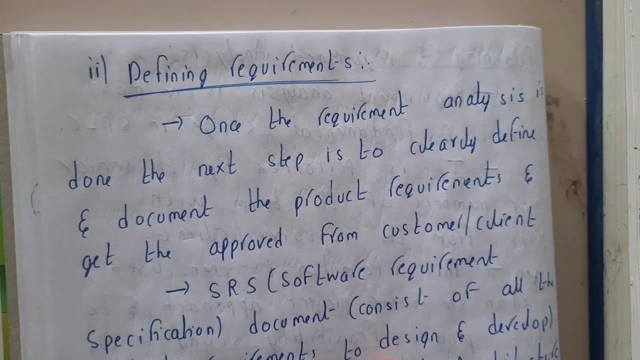 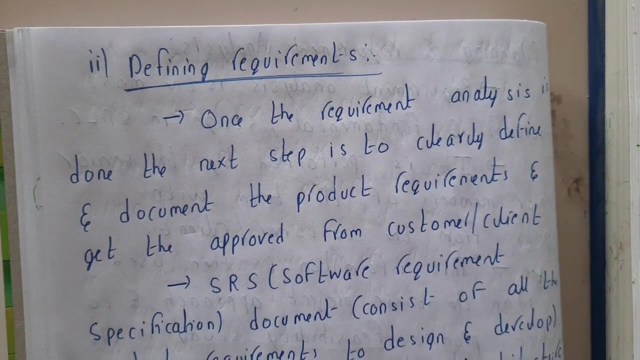 So, once the requirement analysis is done, the next step is to clear the definition or define and document the product requirements to get approval from the customer. So, instead of directly going to the project development or designing, first get an approval from the client so that you can inform him that. okay, this is what we understood. 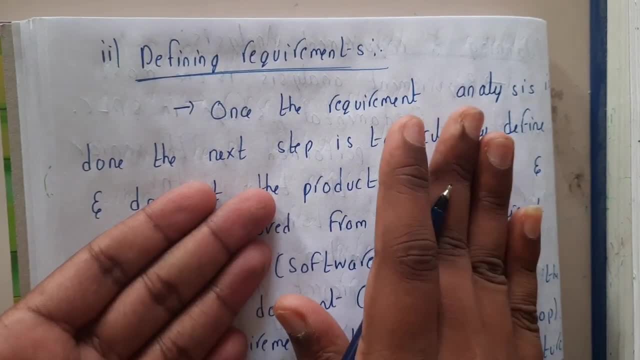 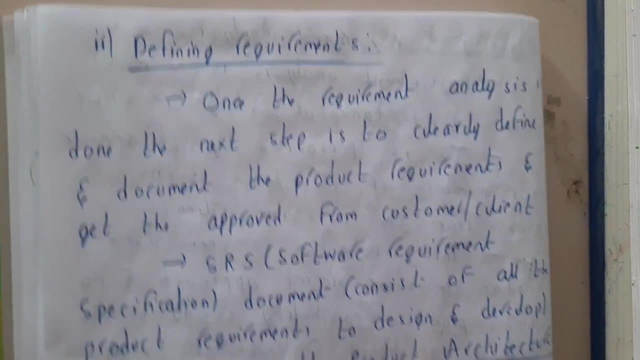 from your requirements. Is this the thing that you want or anything else? If anything, please let us know So that we will change it and we will let you know again. So in that way you will be going Okay, Okay, So you'll be making SRS that is nothing but software requirement specifications, where 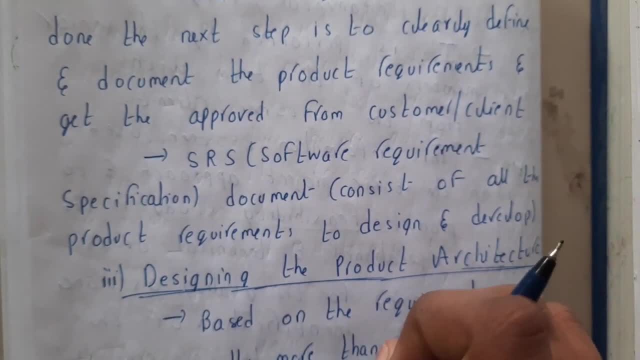 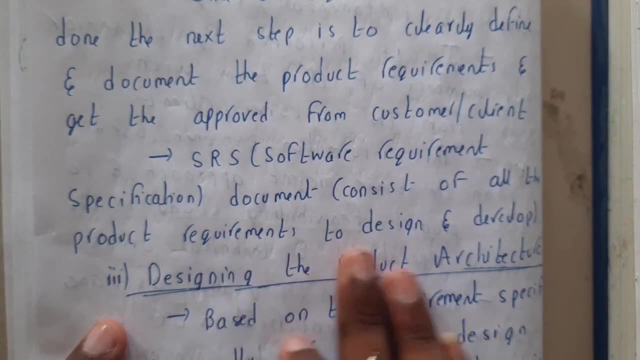 you'll be specifying everything and you'll be doing some basic documentation, because it's not the full fledged documentation. You can say that that is a basic documentation, Okay, And consists of all the project requirements to design and develop- Okay. So basically, in the next step, you will be designing the product. 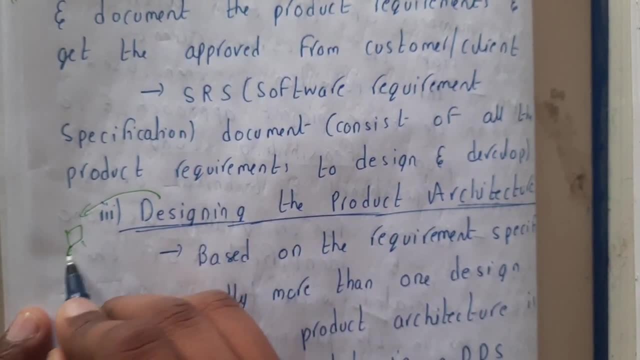 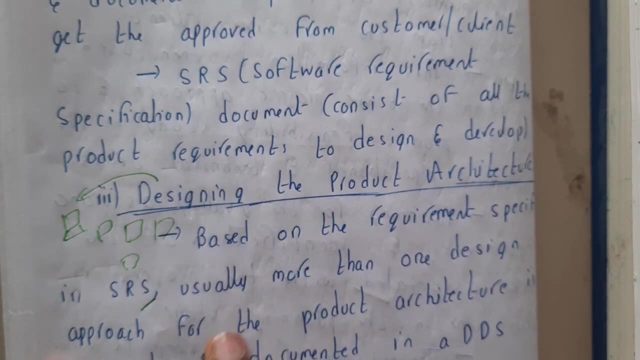 So here you can say that you are designing the product, the outline of the product. So how the product will be, How the modules will be, What, what will be the modules? Okay, So, based on the requirements specified in the SRS, usually more than one design approach is made. 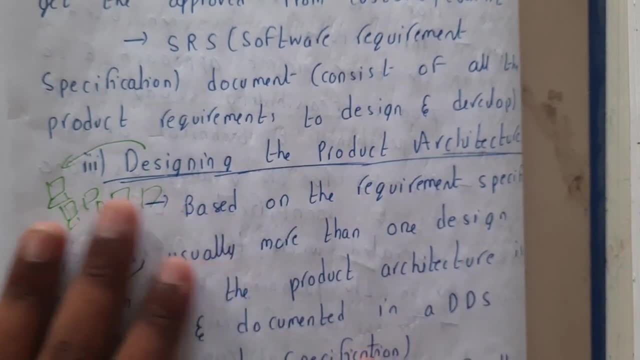 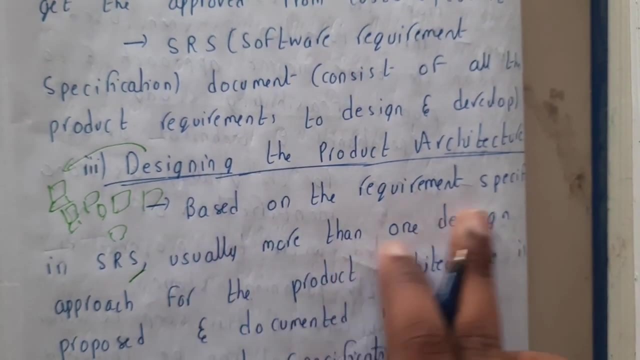 So, basically, you will not make only one design. You'll be making multiple designs, or two to three designs And among those things which you will be deciding, you will be deciding one as a finalist. Okay, So, based on the requirements specified in SRS, usually more than one design approach for a particular. 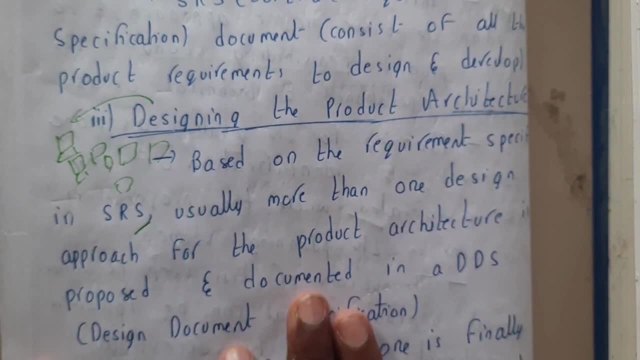 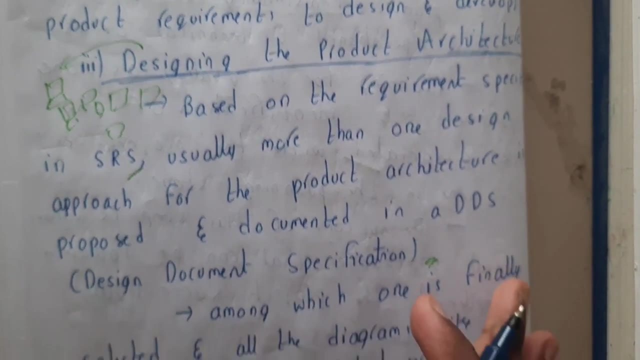 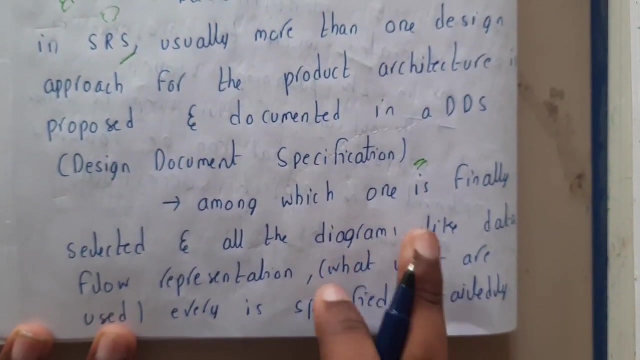 project architecture is made. Okay, So these documentations are called as design documentations. Okay, Okay, So among which one is finally selected, and all the diagrams are like diagrams are represented. What? Okay, Sorry for that. So, basically, they will be drawing some specific diagrams because we'll be discussing about. 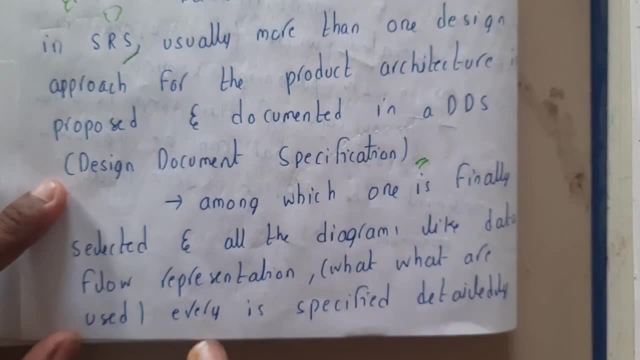 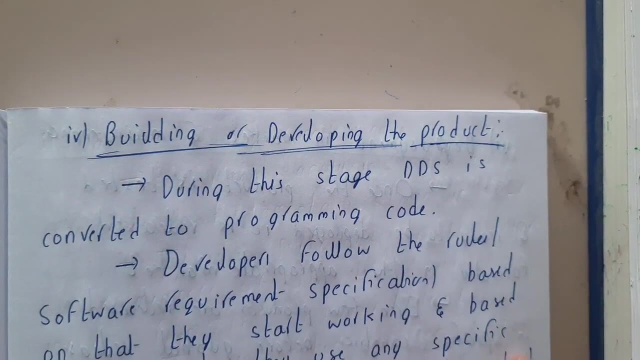 those diagrams also in our later lectures. Don't worry about that. Okay, So everything is specified there. Okay, So after that you will be going to building or deploying the product. They will be calling both the same, Things are same. 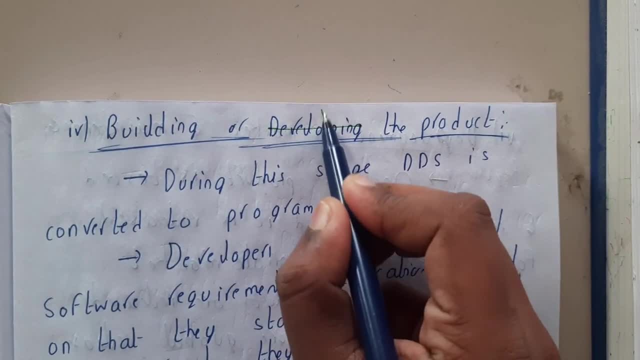 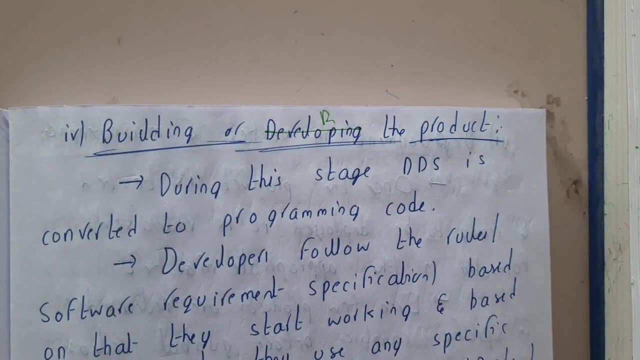 Or you can say: sorry, guys, it should not be deployment, It is developing the product guys. Okay, So in this stage, the finally based on that design, they will start coding guys. So once you assume that, once you design something, coding part will be a hundred percent easy guys. 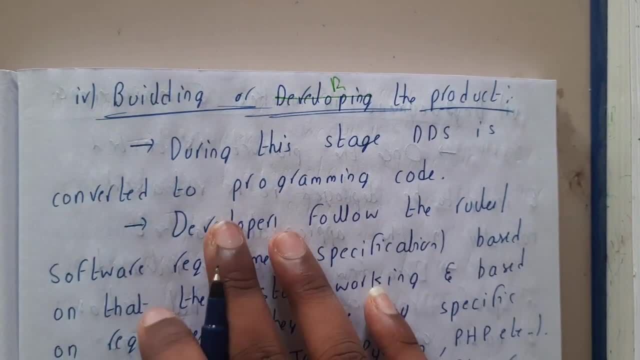 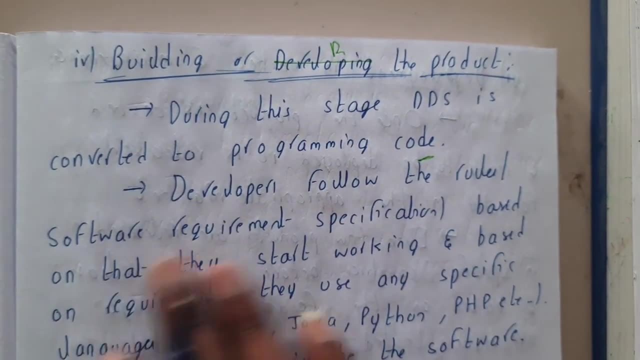 Okay, So during the stage of DDS is converted into programming code. So basically, you will be converting the design into the program. Okay, So developers follow the rules, slash software requirements, specifications. based on that They start working and based on the requirements they use it. 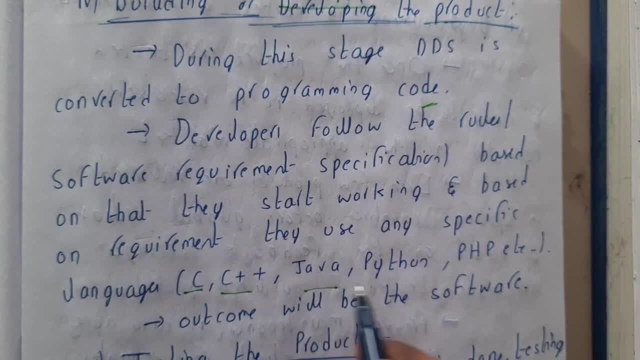 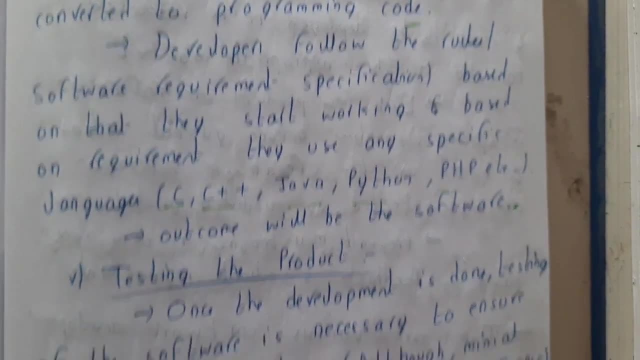 They use a specific programming languages like C, C plus plus Java, Python, PHP, based on the requirements, they will be using the programming language and they will be coming up with the software as an outcome. Okay, So once the pro the software has come out, they will start the testing guys. 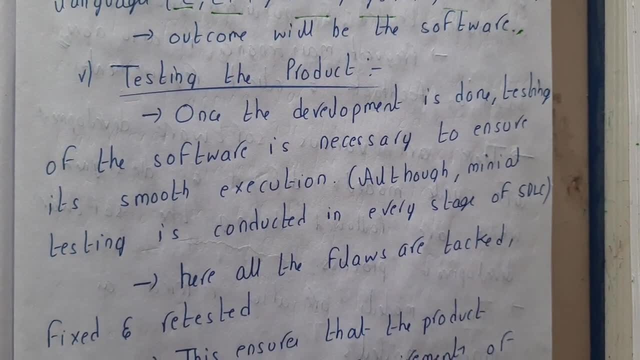 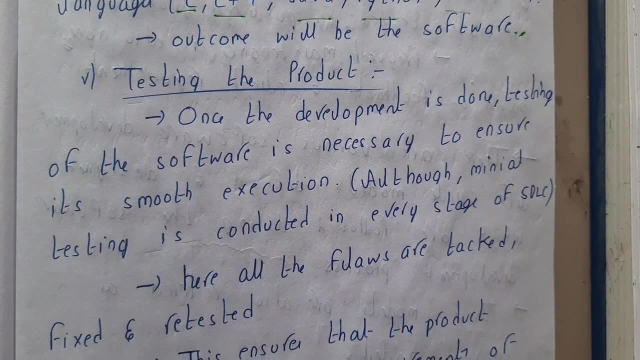 So basically here they will be testing multiple things, like whether it is based on the requirements, whether it is working, whether every module is working perfectly like. they'll be testing it module by module: unit testing, integration testing. There are multiple types of testings. 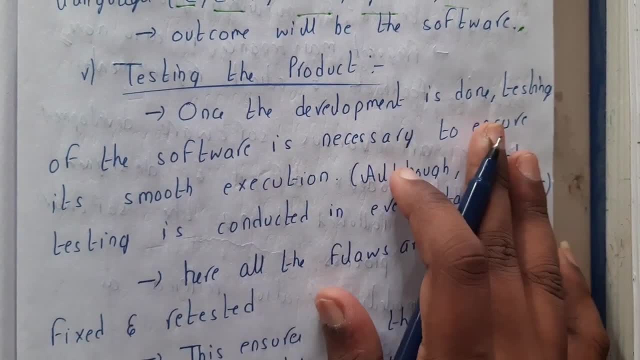 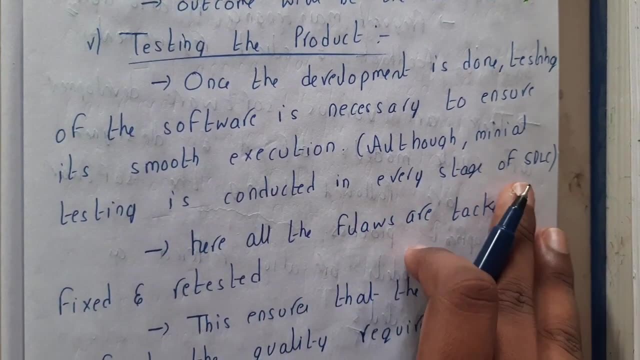 Okay, So once the development is done, testing of the software is necessary to ensure that it is running smoothly, Although minimal testing is conducted at every stage of SDLC, like unit testing and module testing, I told you right. So those are done while building only. 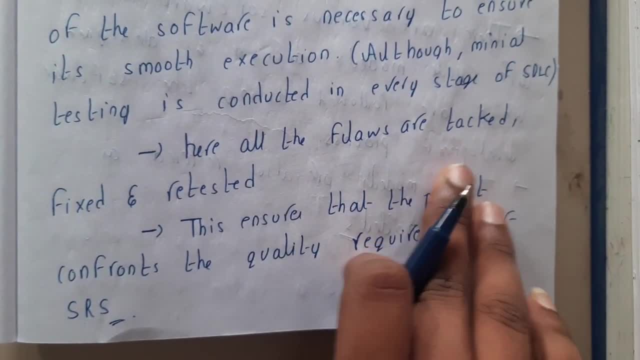 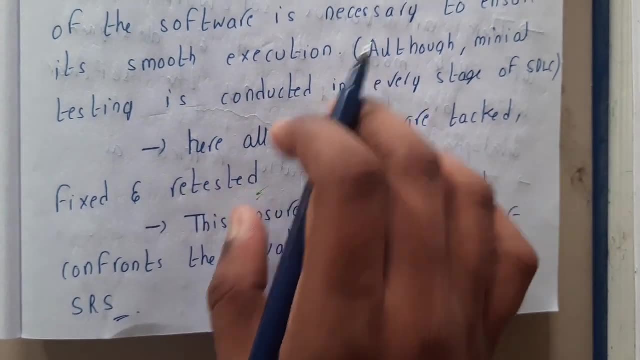 Okay, So here if a flaw are tracked, So if there are any flaws in the code or anything found, they will be testing it and they will be debugging and they'll be resolving it, guys. Okay, So this ensures that the product is confirmed. 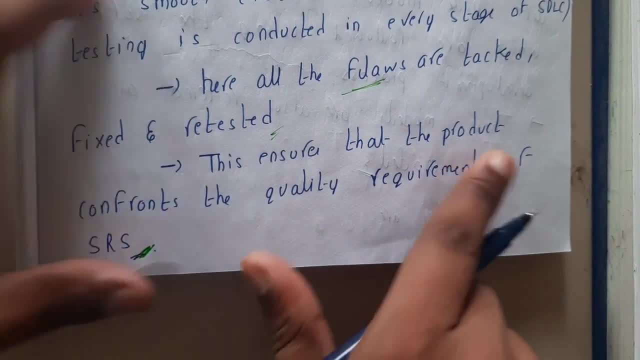 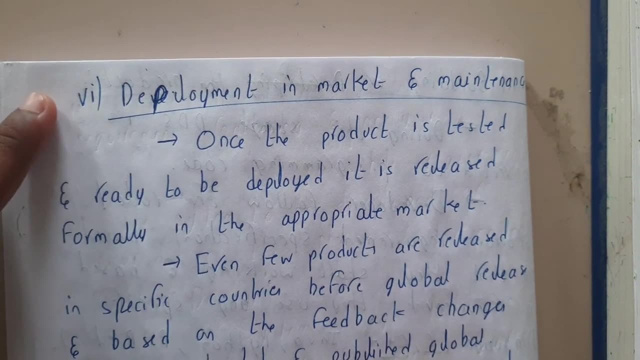 Okay, So after that you'll be solving the SRS. So that is nothing but the requirements. So we will be ensuring that the software requirements of the client have been initialized, Okay, Okay. So after that you will be moving on to development in, or deployment in, market and maintenance. 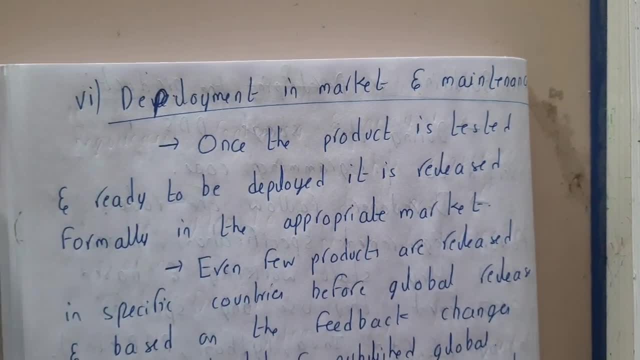 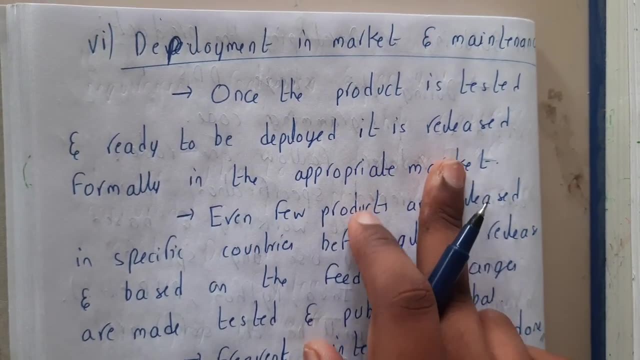 So basically, these are the steps at the end of the project, guys. So you completed the project and now you want to deploy it to the real world. So once the project is tested and ready to deploy, it is released formally in the upcoming months.